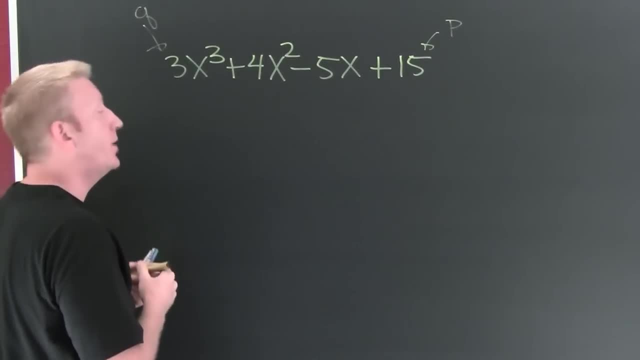 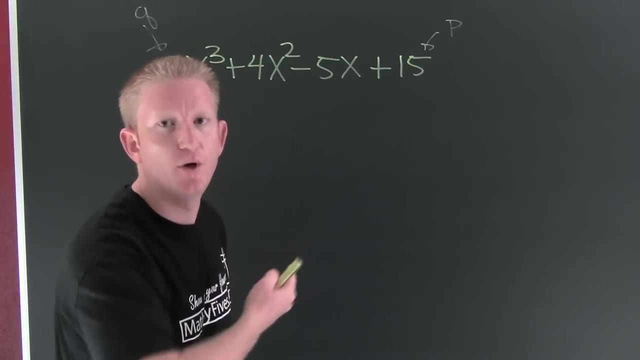 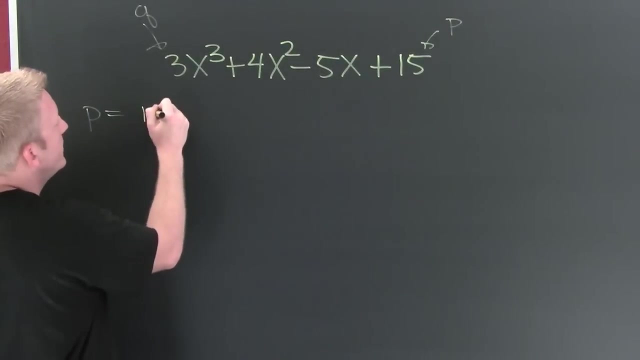 Because the possible divisors for our polynomial, if it's going to divide it, even with a rational number, it's going to be the quotient of p over q, Okay, or the factors of them. So then my p, see my p factors, those are going to be 1,, 3, 5.. 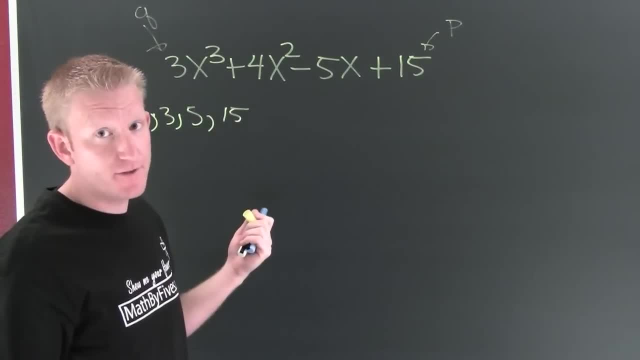 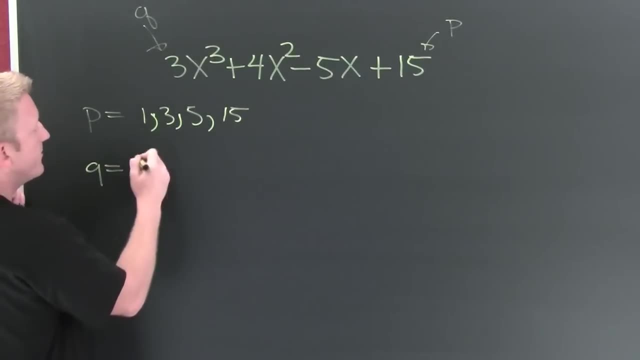 And What? 15.. Are those all the factors of 15? Yes, My q factors, my q Mm-hmm, That's going to be 3 and say 1.. Those are the factors of my q. 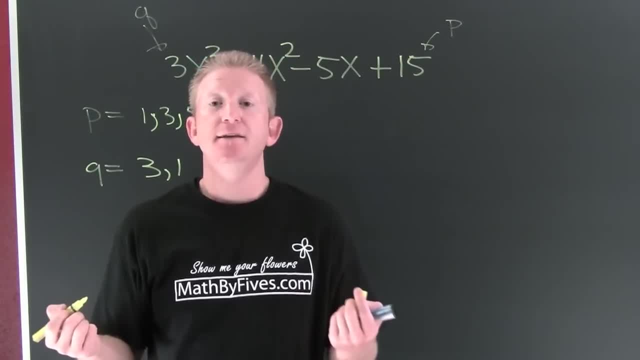 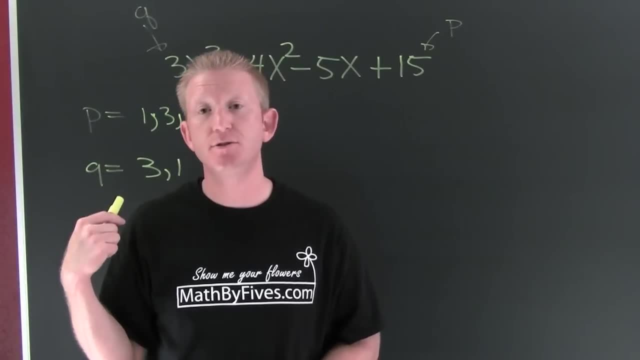 Okay, so what am I going to do? I'm going to go and I'm going to write. I'm going to list the factors of p over q. Why do I want to do this? Yeah, because I want to try to factor this thing using division, because I may not have the skills and techniques to. 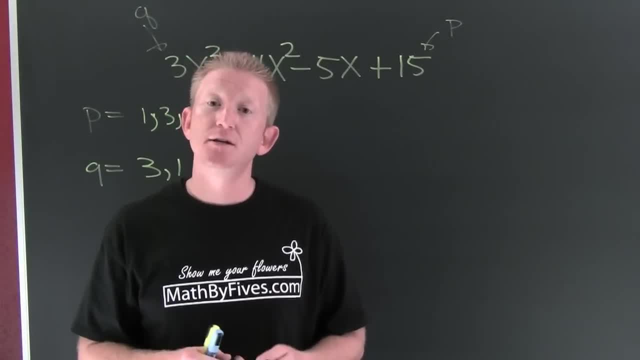 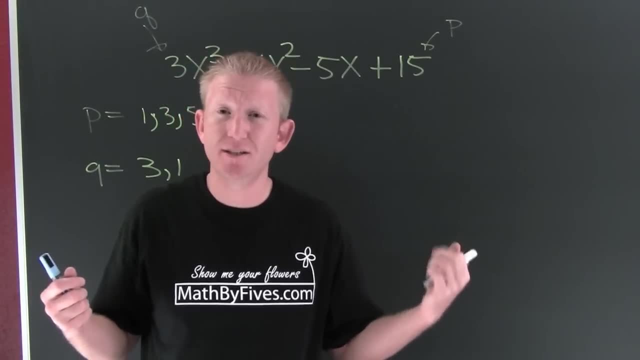 Okay, Yeah, factor it by the traditional methods. So I want to factor by division, So I need possible divisors. and what are they going to be? They're going to be the quotients of p over q. You're going to say this is an awfully long list, but hey, it's a lot shorter than all the numbers in the entire world. 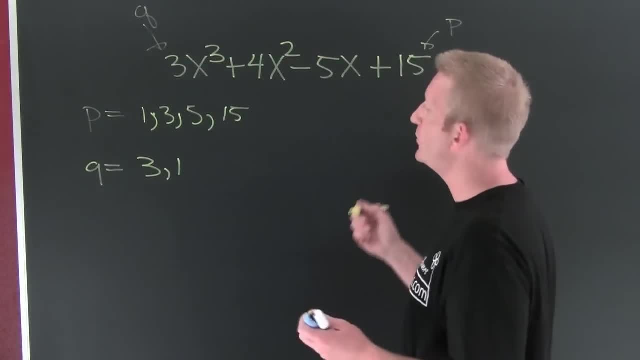 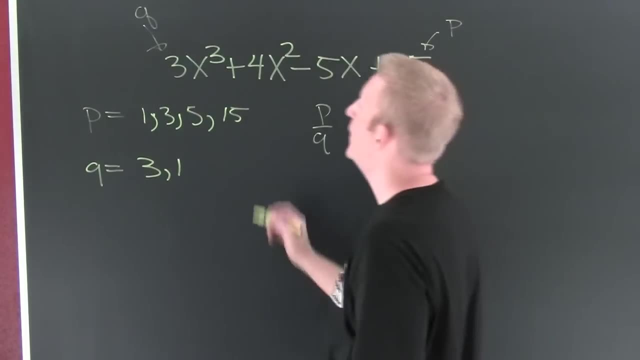 So let's get at it, people. Mm-hmm. Okay, so I'm looking for p over q. Yes, So then why don't I just fix a q? Sure, Here I'm going to fix a q. Let me let q be 3.. 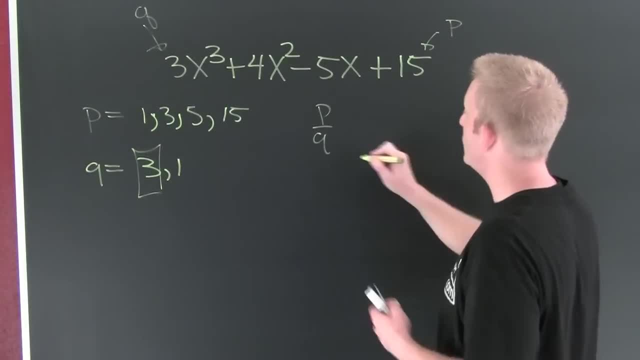 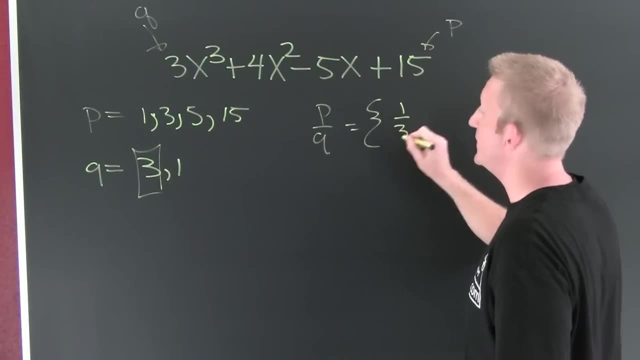 Okay, So I'm going to take All of these and I'm going to divide them by 3.. So in my list, in my list of potential divisors, I'm going to have 1 over 3.. I'm going to have 3 over 3.. 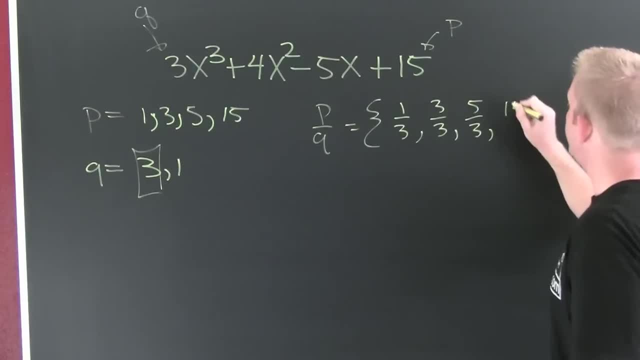 I'm going to have 5 over 3. And I'm going to have 15 over 3.. Okay, So now that I've exhausted 3, let me fix my q now to be 1. The other potential denominator in my rational. 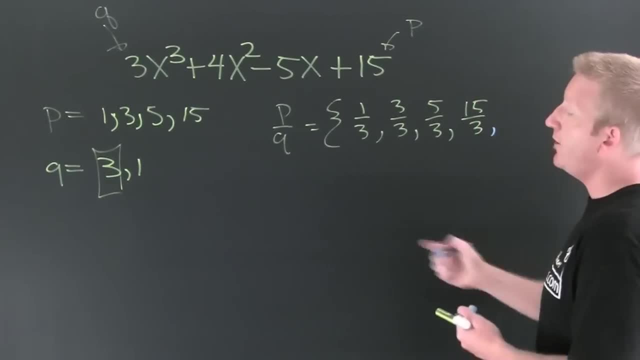 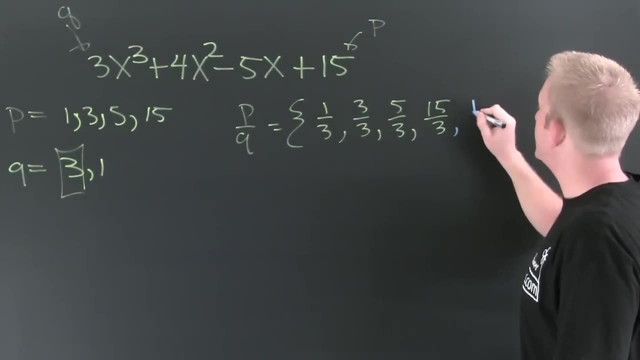 Factors, if there are any. yeah, um, now I've fixed q to be 1, so I'm going to take all my p's and divide them by all my q's. Here we go. That's 1 over 1..